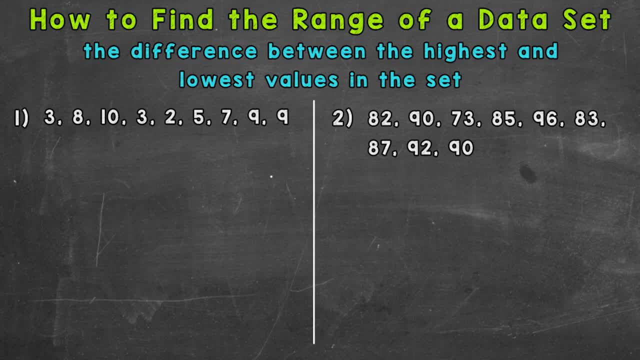 one. So for number one we have a data set that is out of order, So the first thing we want to do is put it in order from least to greatest. That's going to help organize us and also make it much easier to calculate range once we get to that point. So the first number, the lowest valued. 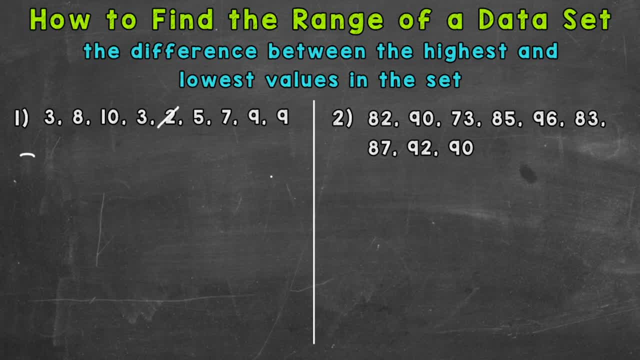 number within that set is two, So I put my two. Then we have two, threes, And I'm crossing those numbers off as I go along. That way I don't miss anything and I don't count anything twice. Then we have a five, a seven, an eight, two nines and lastly a ten. So now we are ready to. 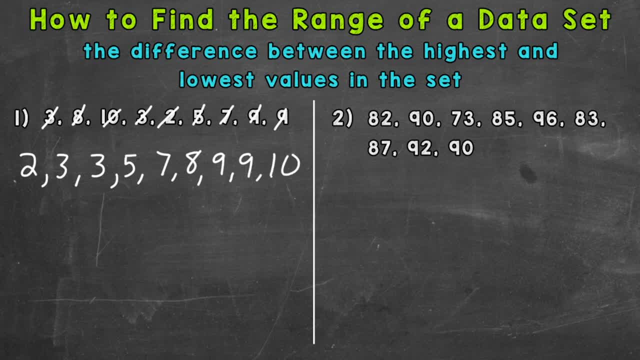 calculate range And we do that by finding the difference between the highest and lowest values in the set. That will give us our range or distance between our highest number and our highest value. So let's do that. So our range is 10 and our lowest is 2. So we would do 10 minus 2. That gives us 8.. 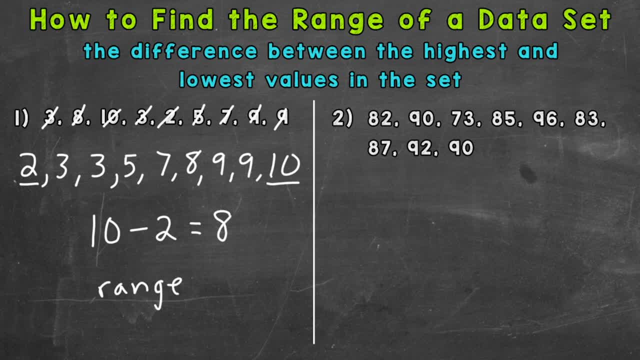 And that is our range. So our range equals 8.. All right On to number two. here Again, this data set is not in order, So let's put it in order from least to greatest, And our least valued number here is 73. Then we have an 82,, 83,. 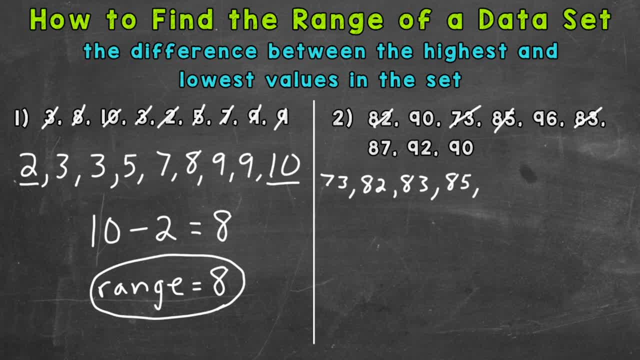 85,, 87,, two nineties and then a 92. And lastly 96. So we take the difference between the highest and lowest values in that set in order to get the range. So our highest is 96. And our lowest is 73. So we need to do 96 minus 73. And that will give us our range or distance.